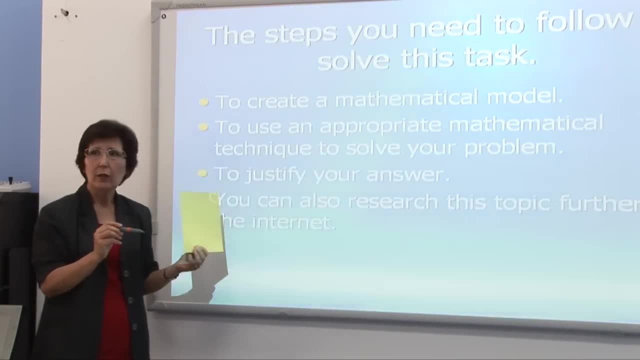 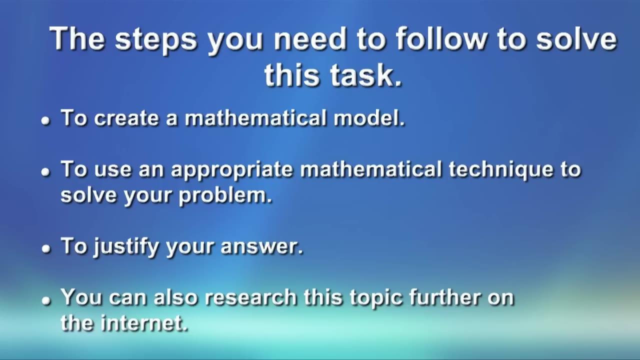 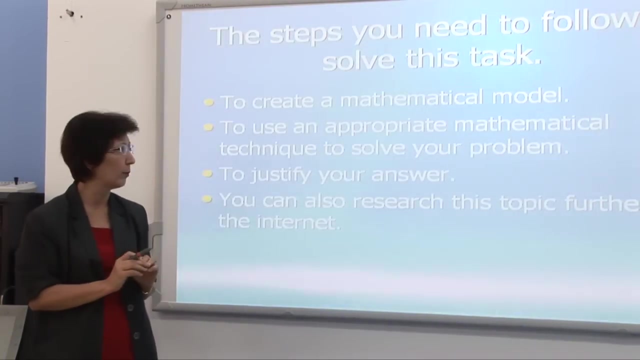 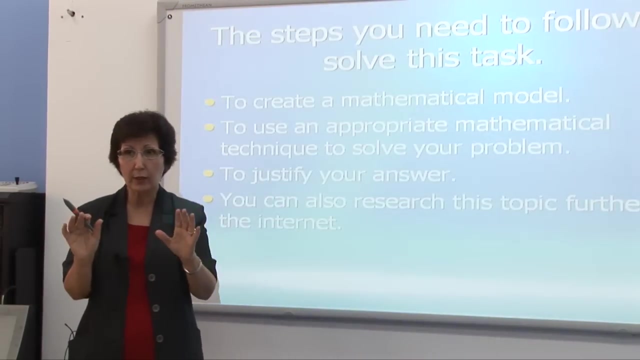 practical problem. First of all, you have to make a mathematical model out of this practical situation. Afterwards, you need to find an appropriate mathematical technique in order to solve the problem. Thirdly, you obviously have to use mathematics again to justify your answer. 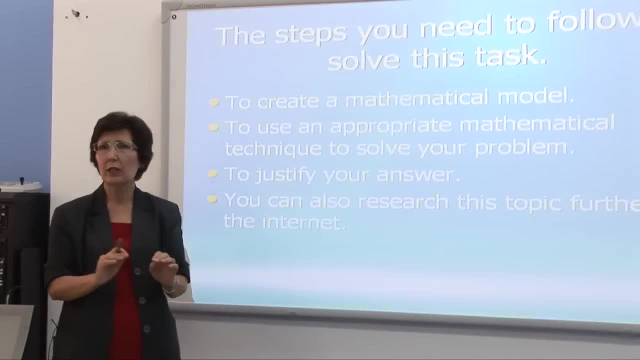 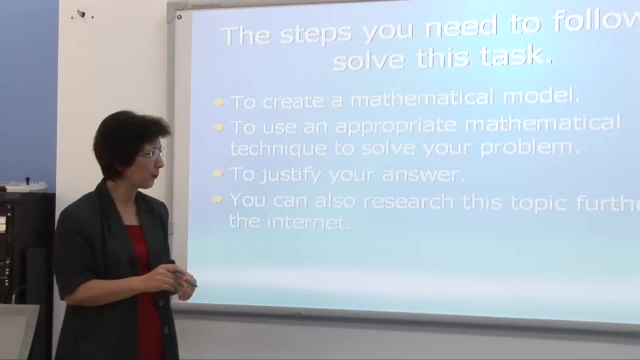 And in doing all these, you can obviously refer to Internet. Sky is the limit and you can find loads of information. Now, how do we make a mathematical model out of this? I have a car in my home and I have two cars on the highway. 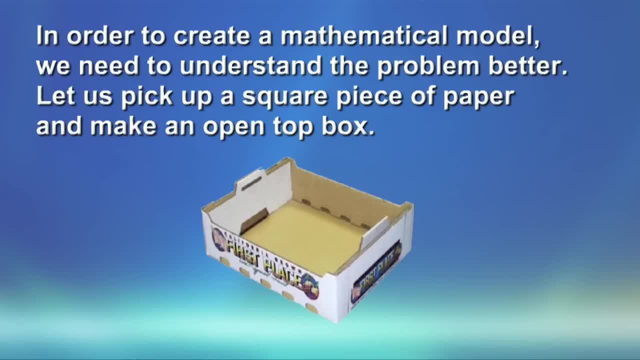 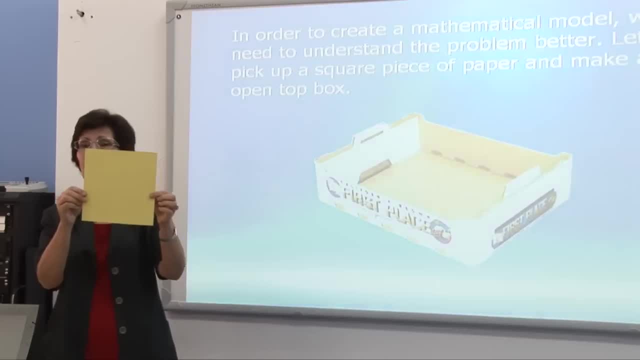 So this is a car that is going to be in my car. I have a car with two drivers and I have two cars that will start heading to my car. cardboard box, cardboard piece of paper, and I want to make a box out of this. 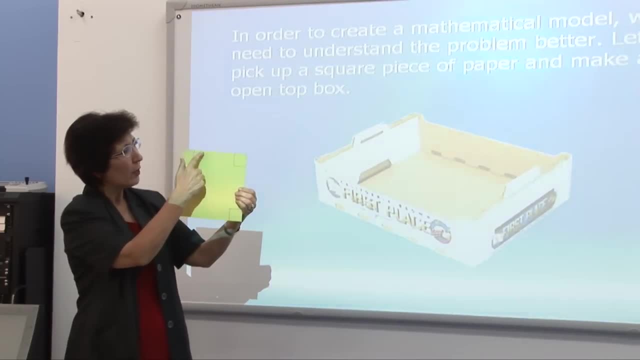 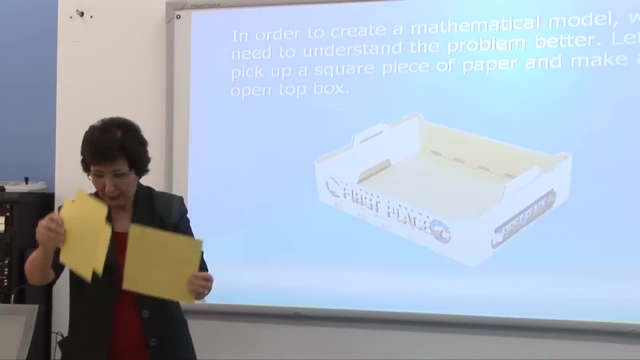 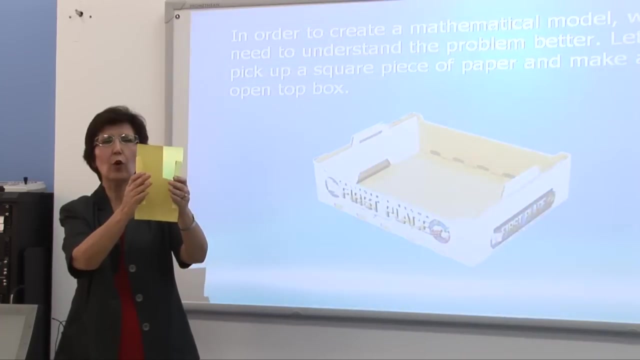 The first thing I do: I make four corners, four squares in each corner, Then I cut them off, which you have something like this. Then, obviously, you fold these like these and by doing that, you will end up with a box Pending on what size square you are going to cut from each corner. you 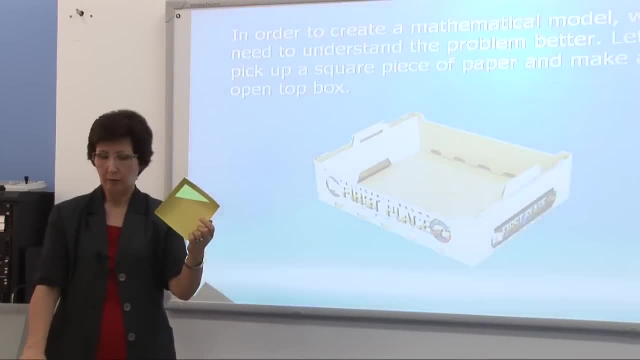 will end up with different sized boxes. If you cut a small square, you will have a box like this, a wide box. If you cut a bigger square, you will have a smaller square like this, a big square. Then, if you cut small square, 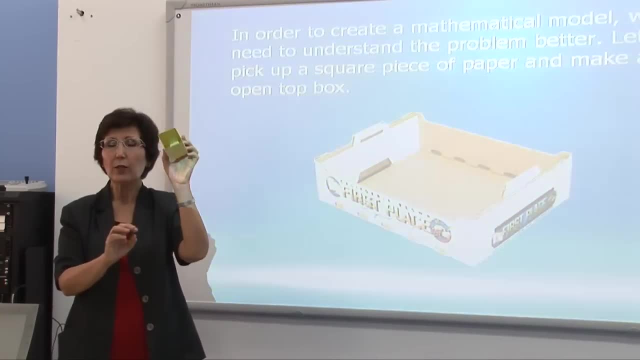 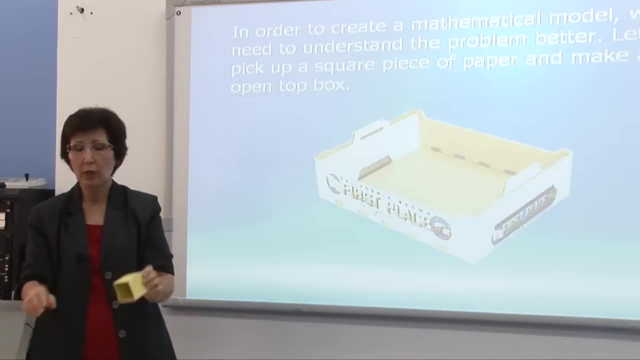 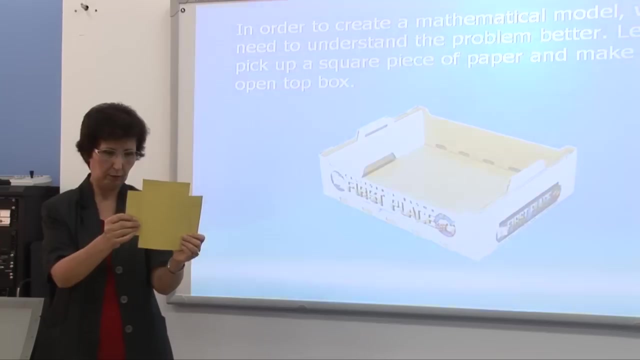 you will have a box like this, But we are interested in the box with the maximum volume. So what we try to do, we try to find a function for the volume of this box. How do we do that? Obviously, if I look at this one, when you cut it and you 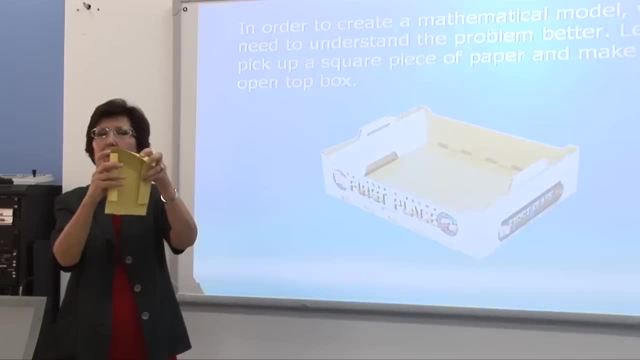 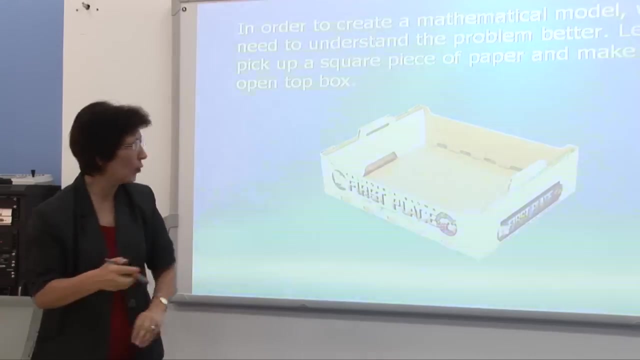 make the box like this: this cut becomes the height of your box and this one, if you look at this, is really the length of this side minus twice, whatever this is. So, if I go into a mathematical model, okay, ok, going in. 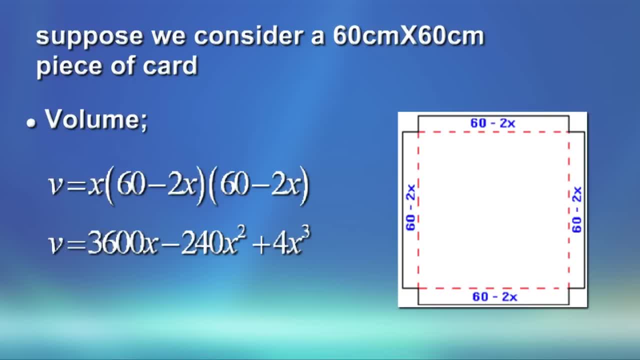 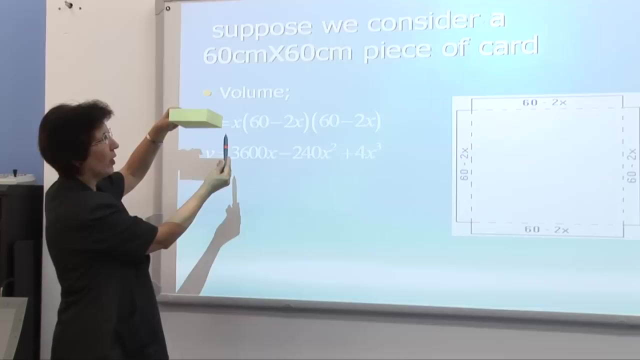 is my paper and, in order to make it simple, I'm going to look at a specific size paper- 60 by 60- and I am assuming that I'm cutting off square which is x by x. so therefore, I will end up with a box which is 60 minus 2x- 60 minus 2x- as 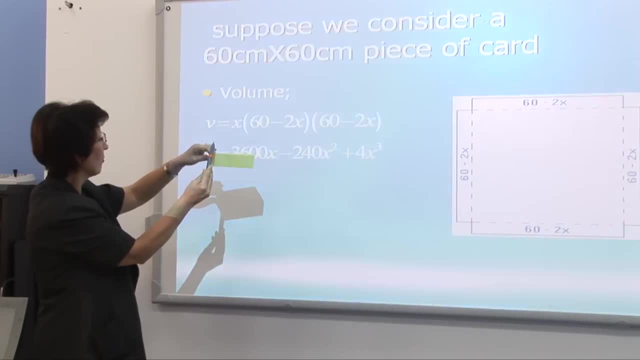 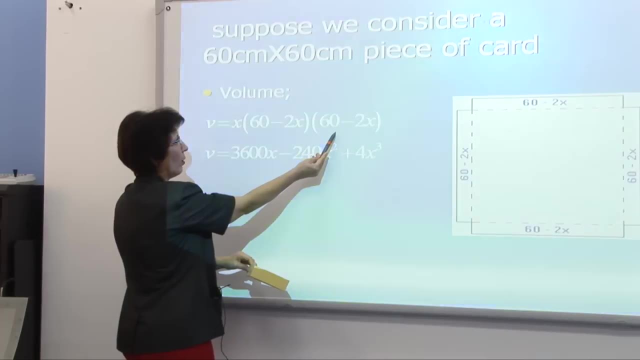 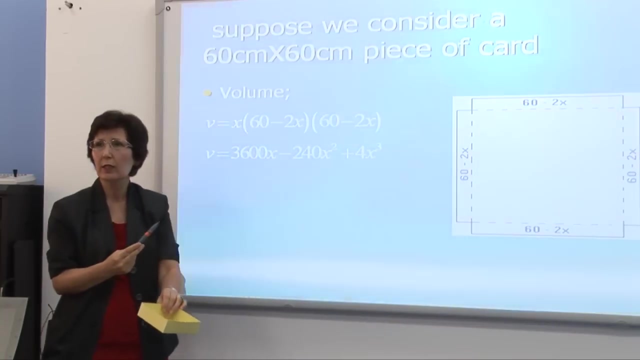 you can see here, and the height is x and the volume can simply be found by the base area: 60 minus 2x, 60 minus 2x times the height, which is x, and if you multiply the brackets together with x outside, you will end up with a function. 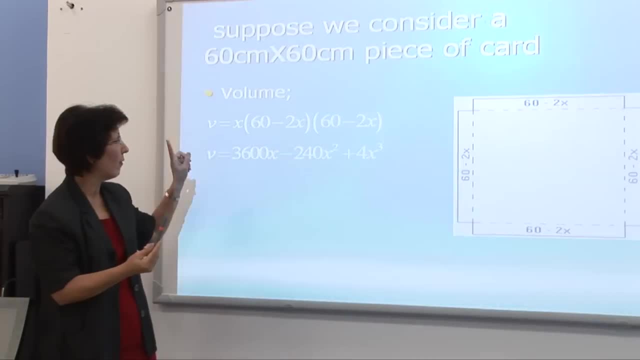 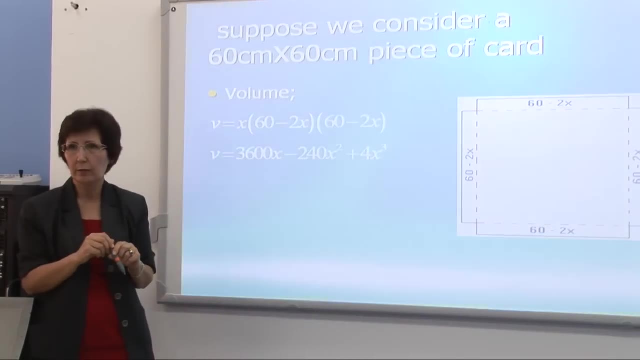 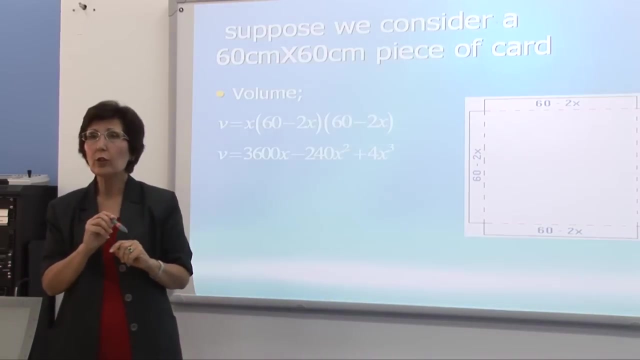 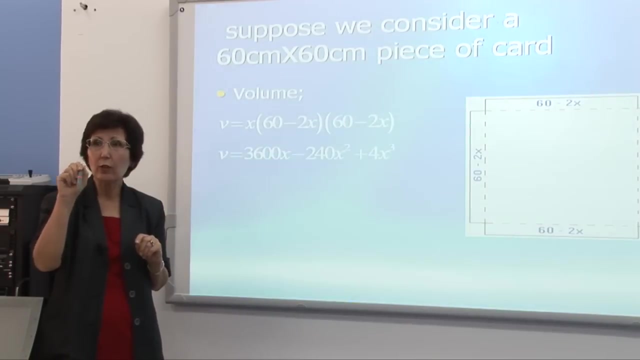 for the volume. Now we want to find the value of x, which makes v maximum x. For this we use calculus. We know, if we find the derivative of a function and equal it to zero, then that will enable us to find the value of the variable. 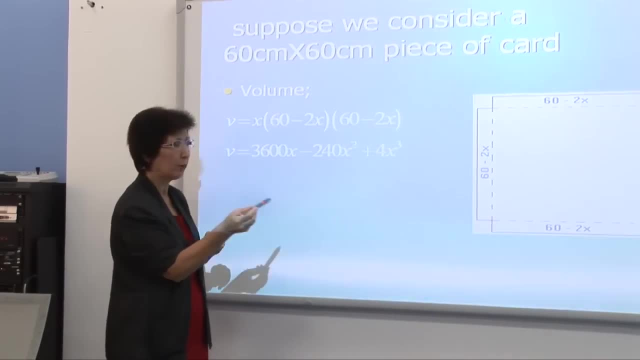 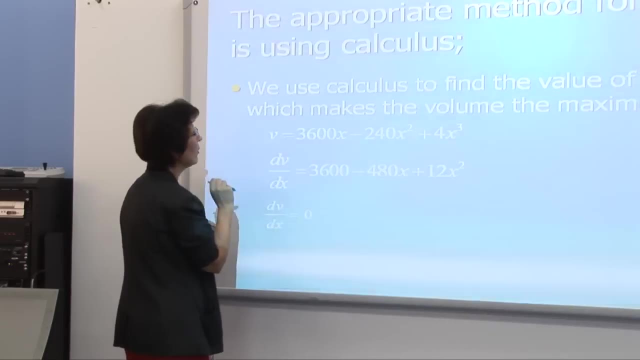 which makes that function maximum or minimum. So what do we do? We have created a problem, we carry on and we are going to solve it. So what do we do? We have created a problem, we carry on and we are going to solve it. So what do we do? We have created a problem, we carry on and we are going to 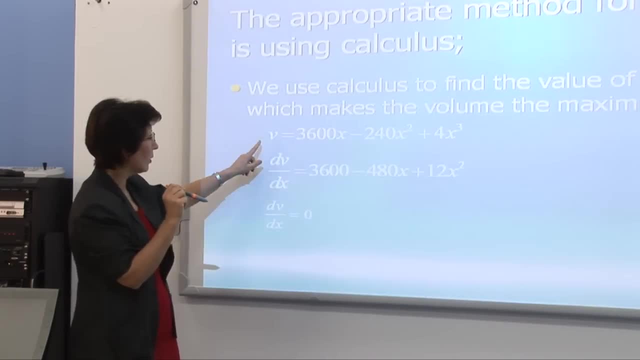 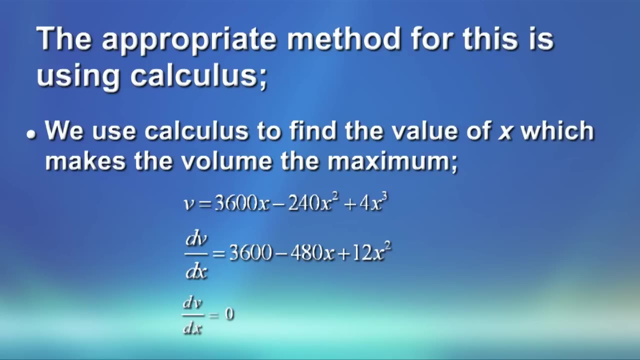 using the calculus. This is our function. we find the derivative in order to find the value of x which makes v maximum. We find the derivative of v and we know the derivative is found by multiplying the power of x by the coefficient reducing the power by one. so it can easily be seen that the derivative is three thousand. 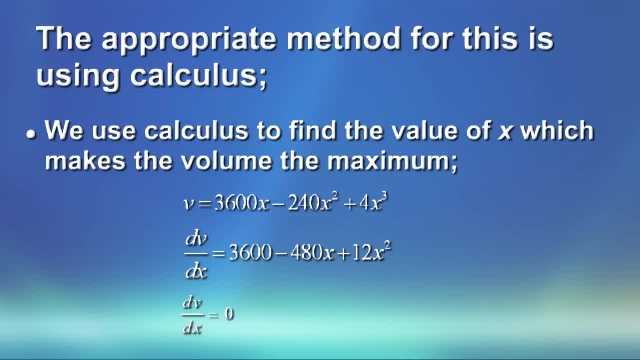 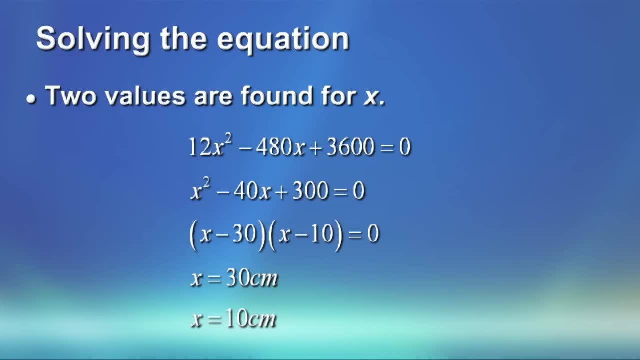 six hundred minus four hundred and eighty x plus twelve x squared, We put the derivative equal to zero and that will give us an equation which, if we solve this equation, we will end up with two values. One value is thirty centimeters. X minus thirty equals zero. X is thirty centimeters. 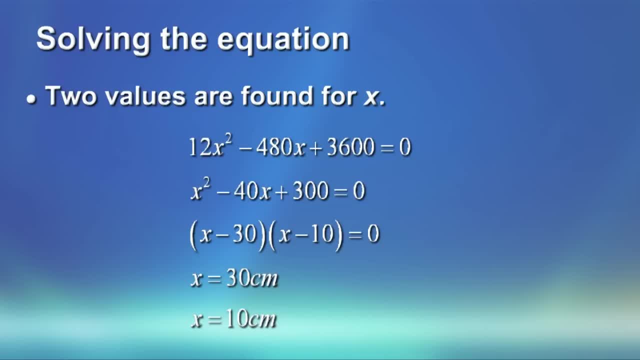 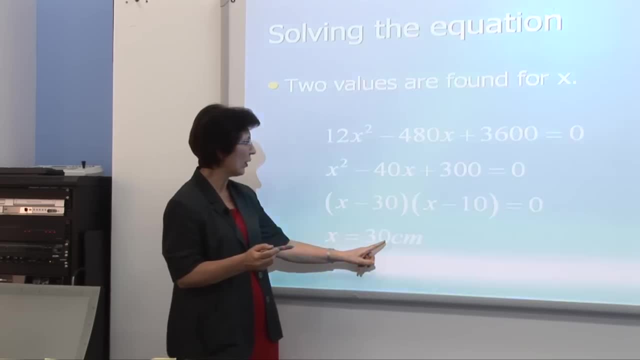 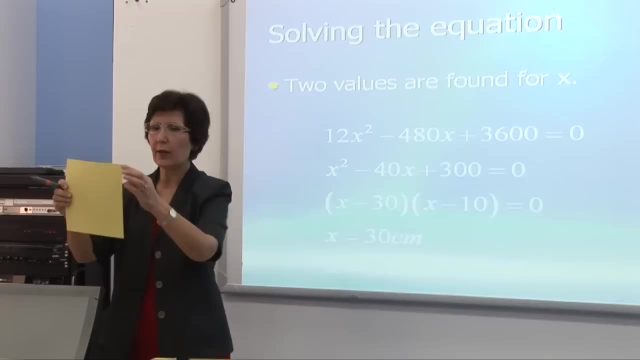 And the other one, x minus ten equals zero, which will give me: x is equal ten. Obviously, x equals thirty is not an appropriate answer, Since the whole size of the paper was sixty. if I'm going to cut square thirty by thirty, I will end up with a volume which is zero. 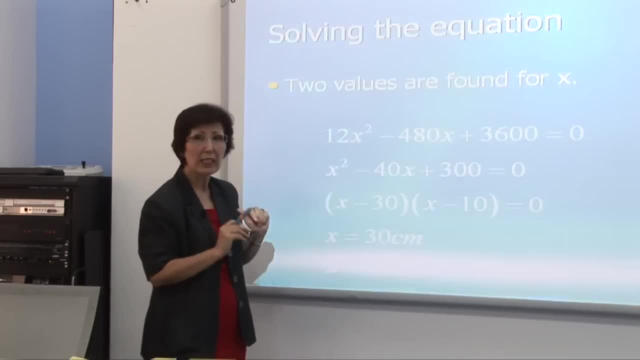 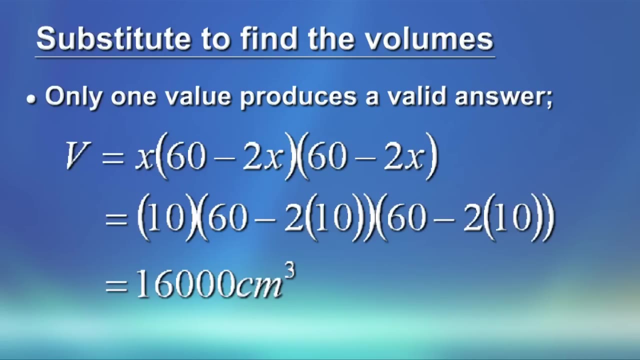 and that's really the minimum value. The one we are interested in is x is equal to ten centimeters and for x equals ten centimeters. if I substituted into the volume function, I will end up with the maximum value of the volume, which you can easily see is sixteen thousand centimeter cubed. 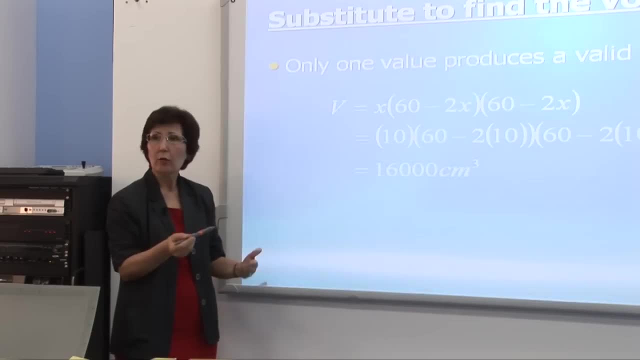 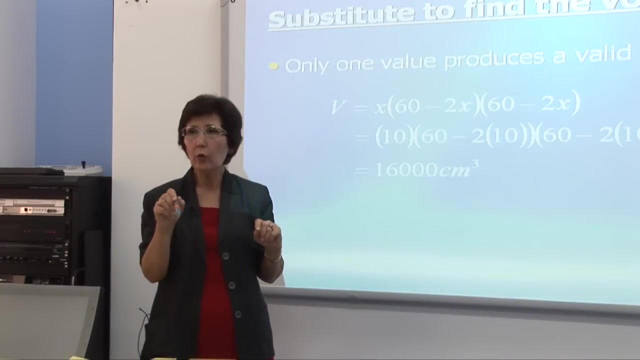 Now, how did this go? How do we know? how can we justify that this is really the maximum value? Again, going back to calculus, we can use the second derivative to justify our answer. We know: if the second derivative for the given value of x is negative, it indicates that 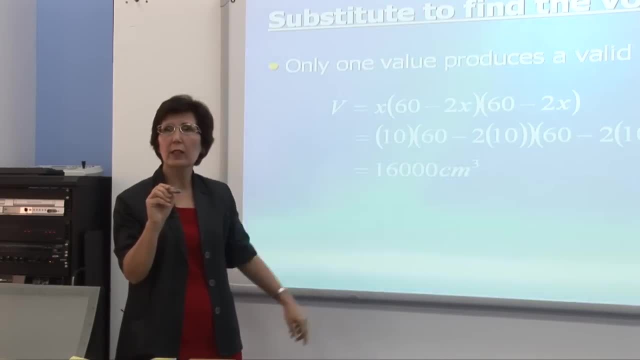 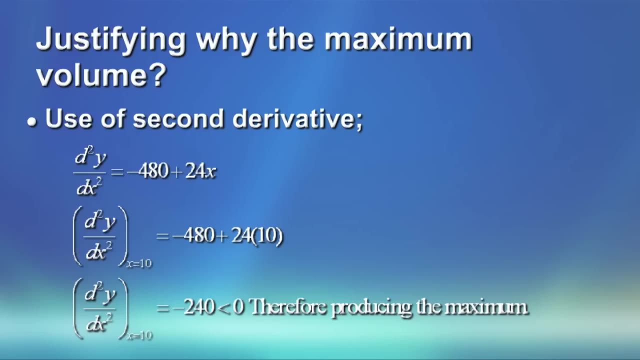 this value of x is providing us with the maximum value. Now, if we go to the next one, we can see the second derivative is minus 480 plus 24x, and if I substitute the value of 10 within this function, you will end up with minus 240,. 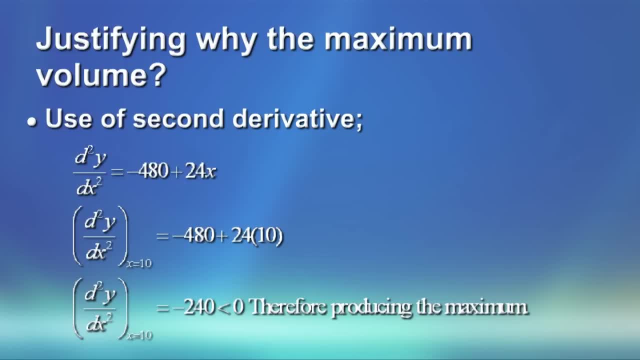 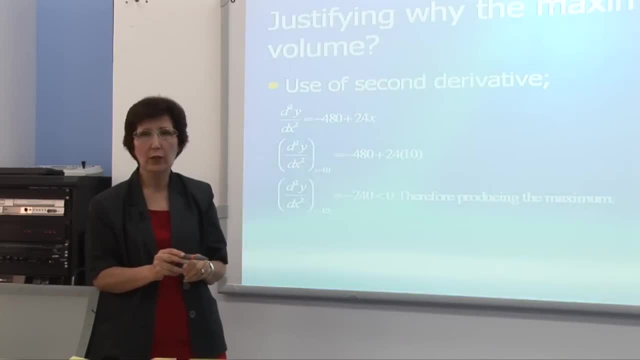 which is a negative value, Indicating that the value x equals 10, providing us with the maximum value for function v.